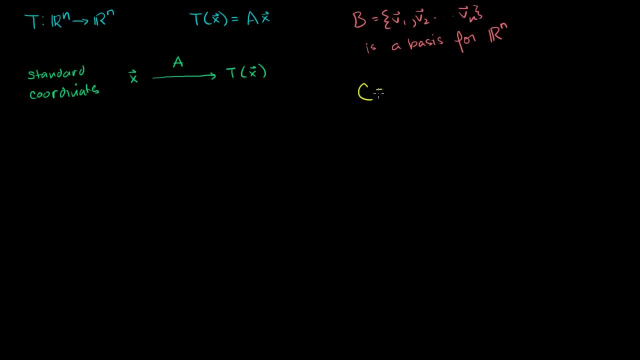 And let's say that C, which just has these guys as its column vectors, C is v1, v2.. All the way to vn Is the change of basis matrix for the basis B. Now we've learned. we've seen this several times already. 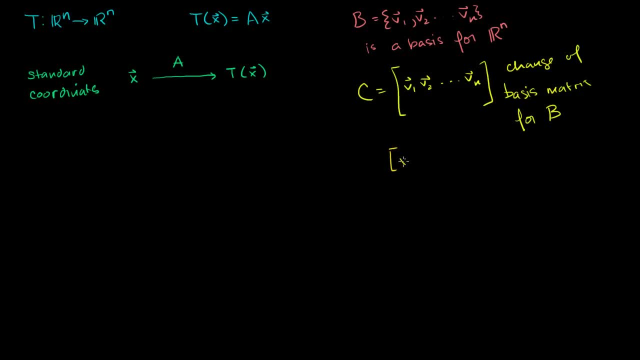 that if I have some vector x in Rn represented in b coordinates or in coordinates with respect to b, I can multiply it by the change of basis. Let's say C is the basis for Rn. Let's say: I have B, so I have B. Let's say I have B. Let's say I have A vector. Let's say I have A vector for B, so let's say I have A vector for B. Let's say I have A vector for B, so I have a vector for Rn, so I 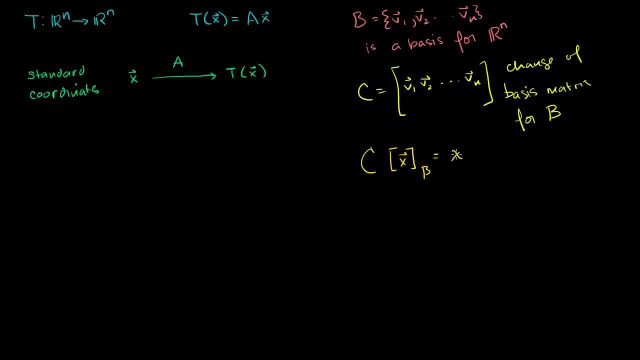 will multiply the vector x, so I'll multiply this matrix, basis matrix, and then I'll get just the standard coordinates for x. Or if you multiply both sides of this equation by c inverse, you can get that if I start with the standard. 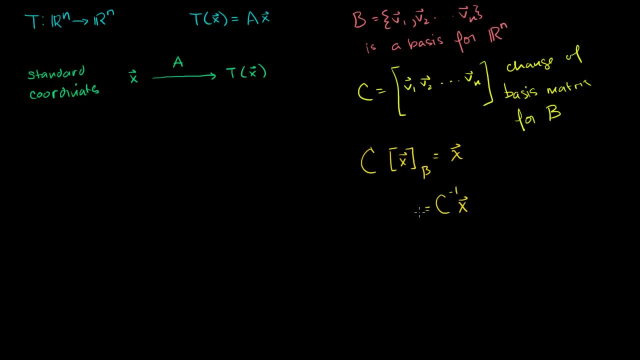 coordinates for x, I can multiply it by c inverse, and then I could get the b coordinates for x or the alternate nonstandard coordinates for x. So we've seen both of these before, so let's apply that to this little diagram here. 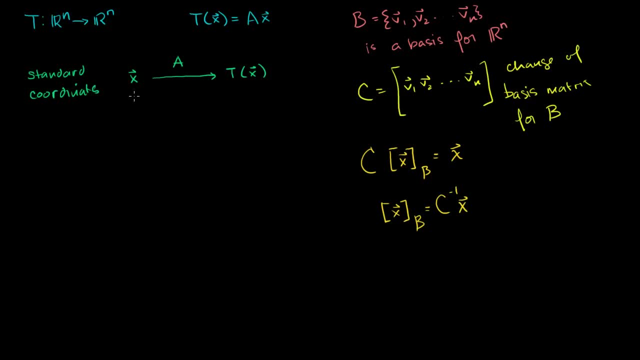 So, if I want to get x and if I wanted to write it in nonstandard coordinates, what do I do? Well, if I have x and if I want to write it, so if I have x, let me go right here. so if I have x, what do I multiply it? 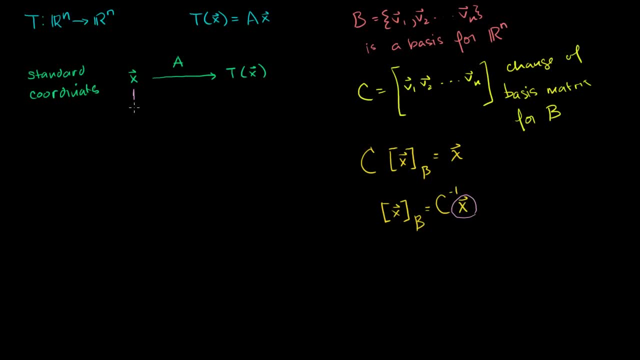 by. if I want to go to nonstandard coordinates, Well, I multiply it by c inverse. If I multiply it by c inverse, whatever I write next to this line, you could say: what matrix do you have to multiply by to get to the end point on your line? 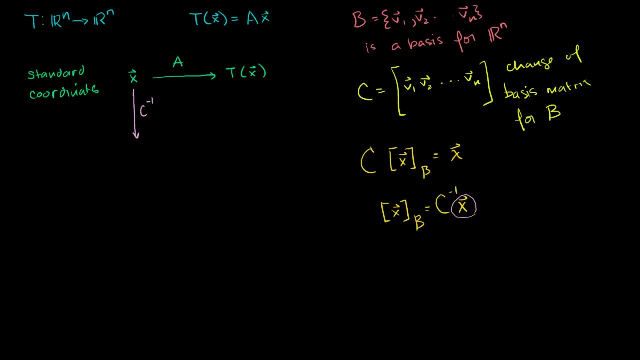 So I multiply x by c inverse, then I get the b coordinates for x. So these are, let's see, coordinates with respect to b. I could do the same thing here with the transformation of x. This is just the standard representation of the. 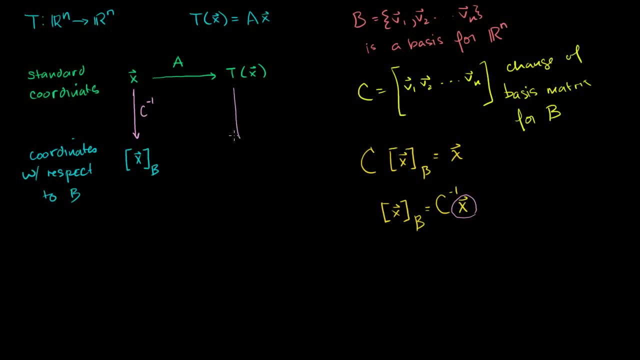 transformation. So I could multiply it by c inverse, if we want to go in that direction, and then we're going to get the transformation of x represented in b coordinates. Now, in the last video, what we saw is: hey, why do these? 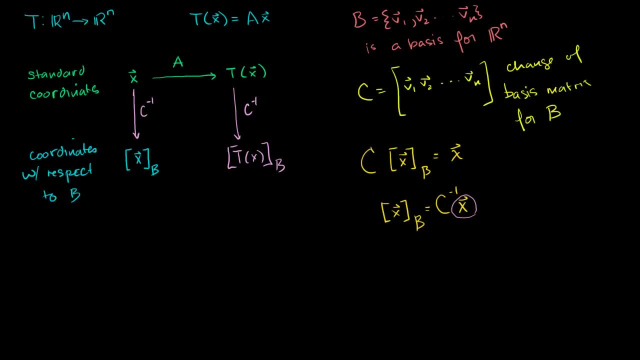 separately. Maybe there is some matrix and we found out what it is. Maybe there's some matrix d that if we multiply this guy times it, I can go straight from the b coordinates of x to the b coordinates of x. So I can go straight from the b coordinates of x to the b. 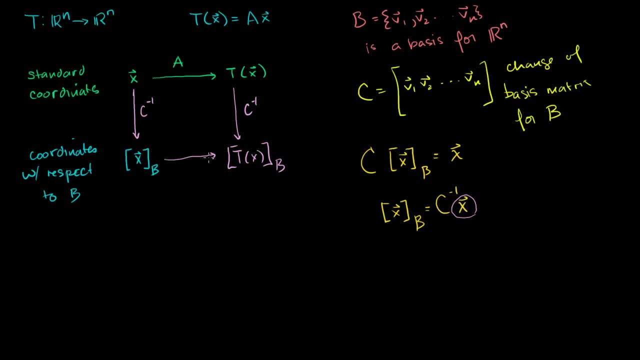 coordinates of x, So I can go straight from the b coordinates of x to the b coordinates of the transformation of x. And we said that is matrix d. And in that last video we showed that d can be represented by a. Actually, you could go around the circle and re-derive it. 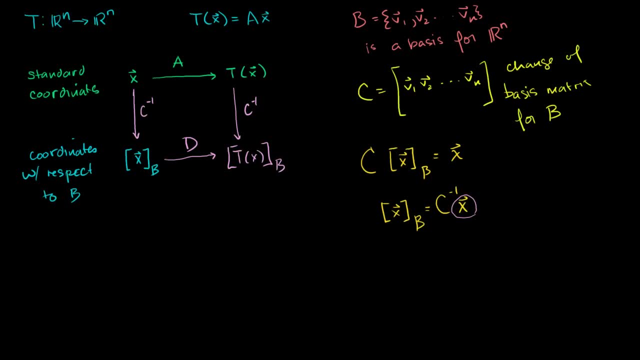 if you like, But we found out that- let me write it in another color- that d is equal to c, inverse times a times c. Now this is all a review of everything that we learned in the last video. Hopefully it clarified things up a little bit. 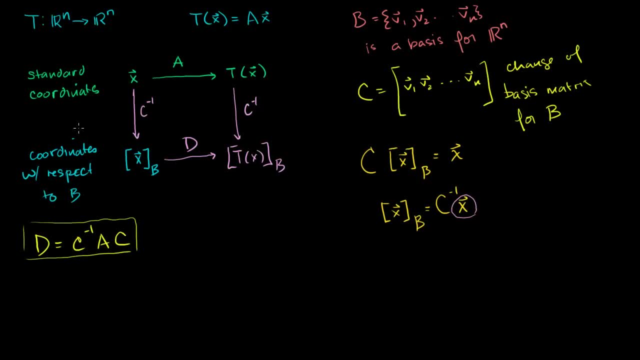 It's nice to just read it, But you realize that these are just alternate ways of doing the same thing. Both of these are the transformation. When you multiply by a, you're applying the same transformation. when you multiply by d, You're just doing it in a different coordinate system. 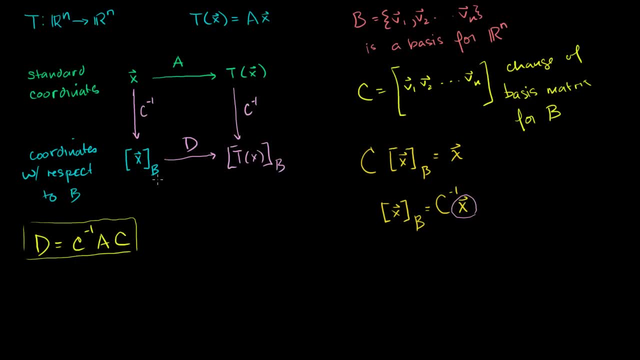 Different coordinate systems are just different ways of representing the same vector. This and this are different labels for the same vector. This and this are different labels for the same vector, So these are both performing the transformation t. Now, this was a relation we got in the last video, that if we 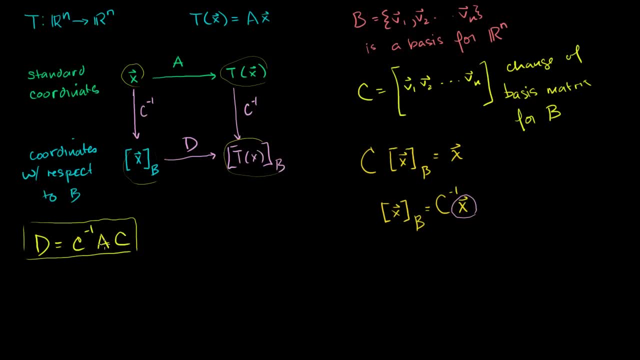 have our change of basis matrix, we have its inverse and we have our standard basis linear transformation matrix. we're able to get this, But let's see if we can go the other way. If we have d, can we solve for a? Well, if you multiply both sides of this equation on the 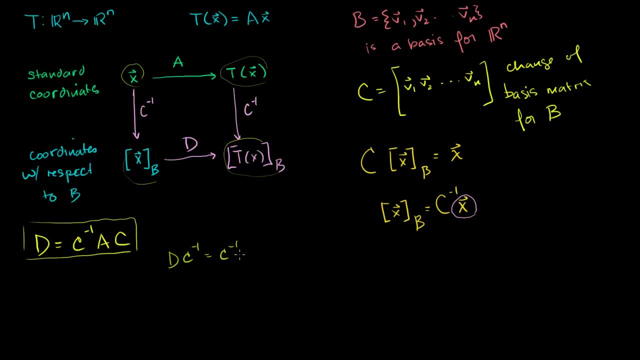 right. by c inverse you get d. c inverse is equal to c inverse, ac c inverse. I did it on the second one. You have a little bit of a distance between here and there. OK, That's fine, I got all the way through. 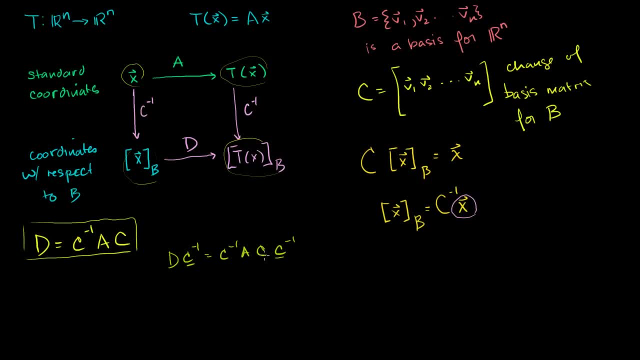 Now it's clear. just put a c inverse on the right-hand side of both sides of this equation. This is going to be the identity matrix, so we can ignore it. And then let's multiply both sides on the left by c, So then you get cdc inverse is equal to cc inverse a. 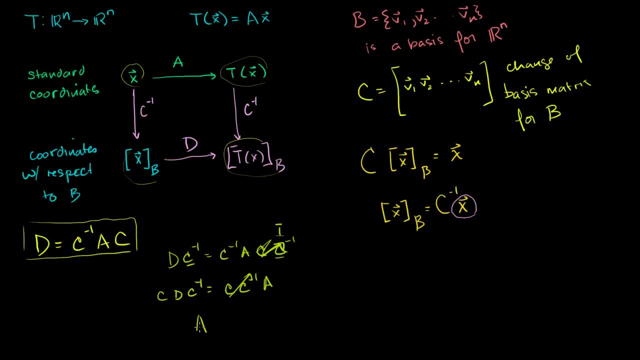 And this is going to be the identity matrix. And then you're left with: a is equal to c times dc inverse, which is another interesting result. It's another thing to put in our toolkit. Now, everything I've been doing has been fairly abstract. 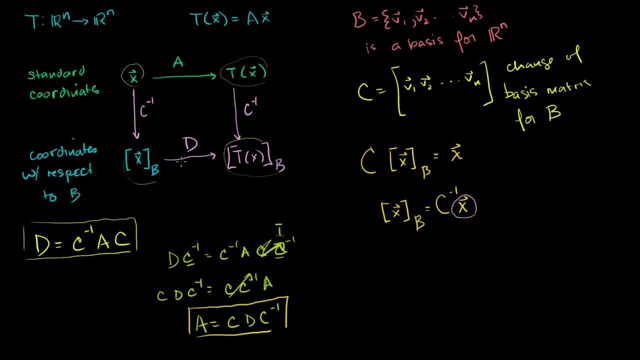 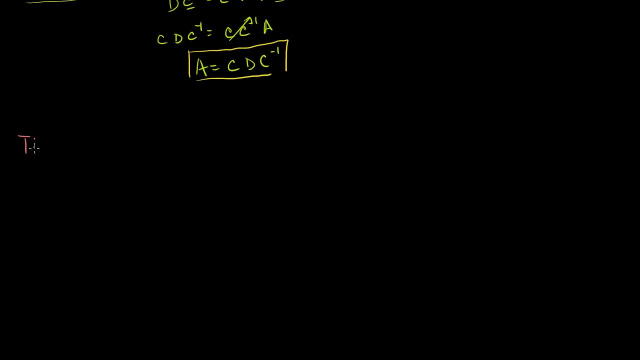 Let's actually apply some of these principles with a real concrete example. So let's say that I have a transformation T. I'll keep these guys around just because they might be useful. That is a mapping from R2 to R2.. And let's say that the transformation matrix for T 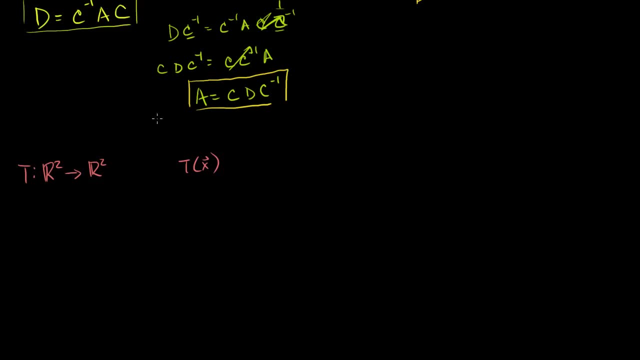 so let's say that T of x- Instead Standard coordinates- is equal to the matrix 3, 2, minus 2, minus 2, minus 2 times x. So this is in the example we just said. this would be our. 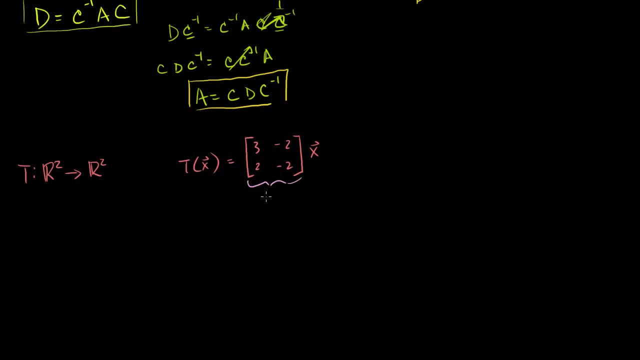 transformation matrix with respect to the standard basis And we could call that a right there. Now let's say we have some alternate basis, Alternate R2 basis. let's call that b, because we've been calling it b so far, And let's say this: alternate R2 basis: the vectors 1,, 2, and 2,. 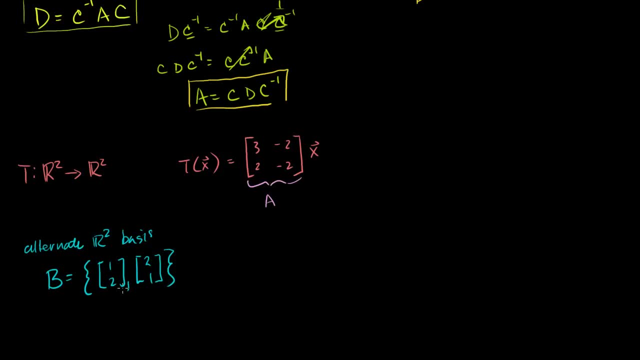 1. So let's see, given this alternate basis, whether we can come up for a transformation matrix in that coordinate world. So what we're looking for? we're looking for some matrix d We're looking for. We're looking for a matrix d such that, if I apply my 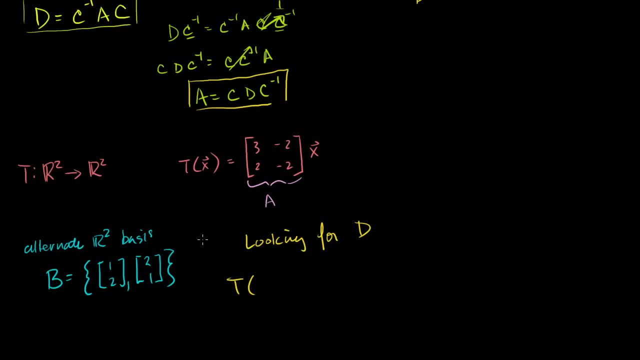 transformation to x in b coordinates. So if I apply it to x in b coordinates or in coordinates, with respect to this alternate basis, it should be equal to this matrix. this matrix, it should be equal to d times x, x in the b coordinates. 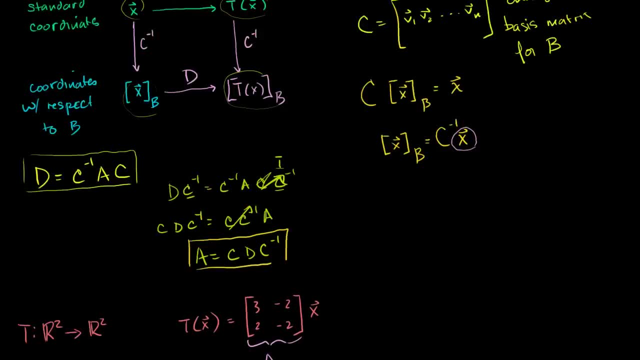 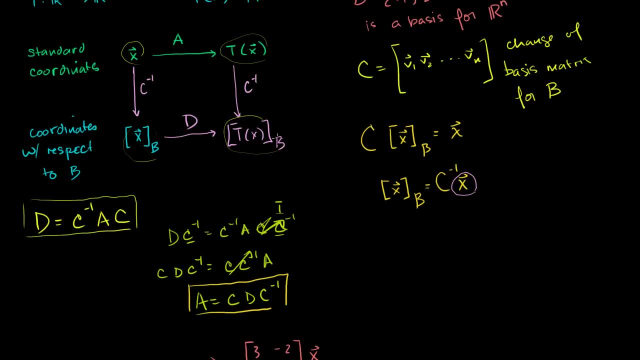 So this is what I'm looking for. I'm looking for that. Or, if we go back to our diagram, I'm looking for that You give me x in b coordinates and you multiply it by d and I'm going to give you the transformation of x in b. 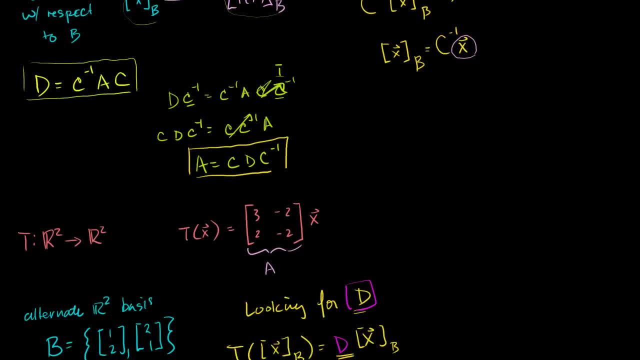 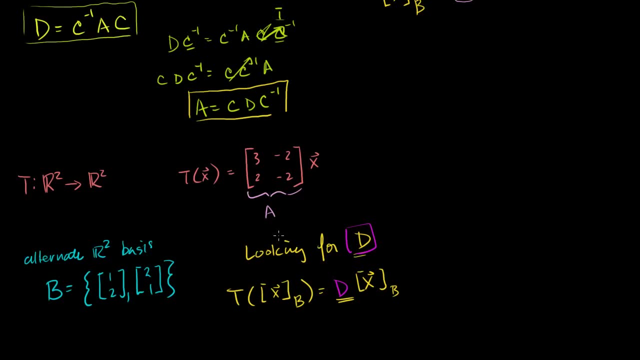 coordinates. Now, just applying it to this concrete example, here we have this formula right here. This is a formula for d, which we proved in the last video. So we have to figure out c inverse. So what is the change of basis matrix for b? 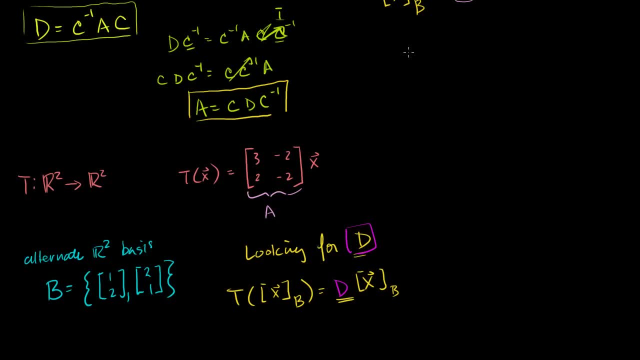 I want to leave this up here. So change of basis matrix for b is just going to be- let's just call it c and it's going to be the basis vectors for b's within the column, So 1, 2, and 2, 1.. 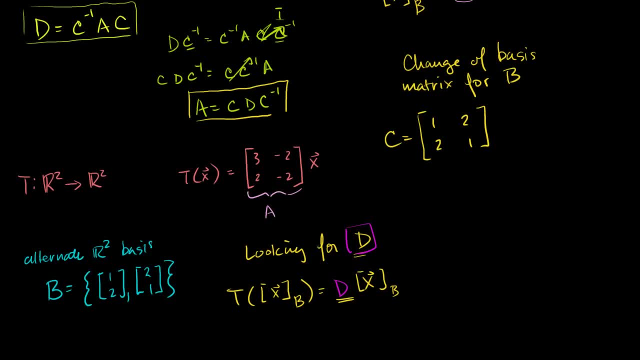 And then we're going to want to figure out its inverse. So let's figure out its determinant first. So the determinant of c is equal to 1 times 1 minus 2 times 2.. So 1 minus 4 is minus 3.. 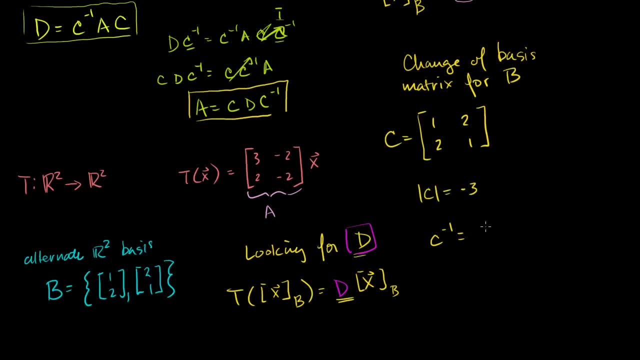 And so c inverse is going to be equal to 1 over the determinant, 1 over minus 3, or minus 1 third times. we switched these two guys. so we switched the 1 and the 1, and then we make these two guys negative. 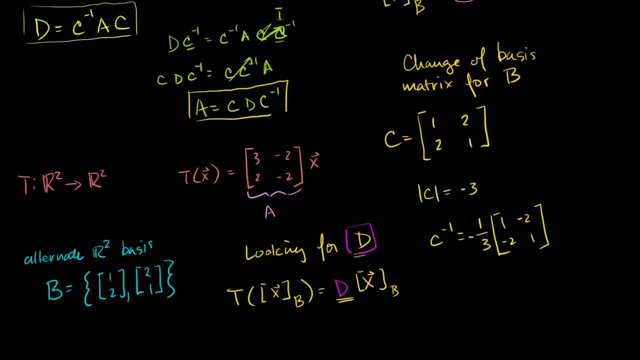 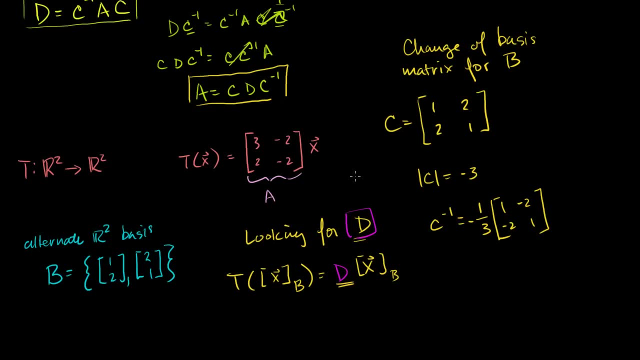 Minus 2, minus 2.. That is c inverse. So d. this d vector right here is going to be equal to c inverse times a Times d Transformation matrix with respect to the standard basis Times c. So let me write it down here: 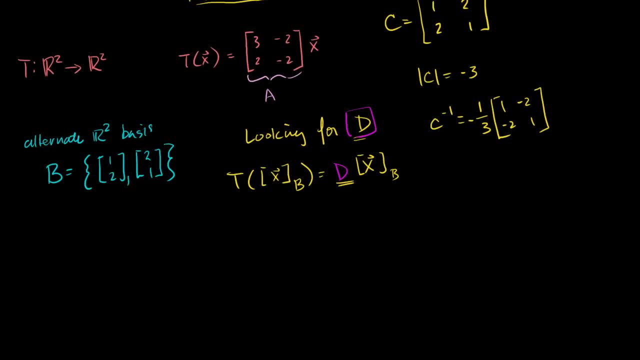 Just because let me write it So: d, the d that we're looking for, d is going to be equal to c inverse times a times c, Which is equal to c inverse is minus 1, third times 1 minus 2, minus 2, 1.. 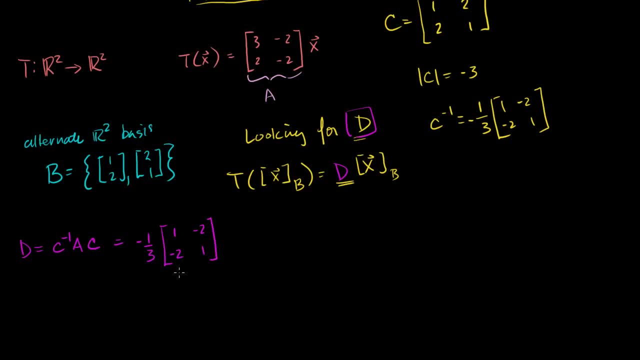 Times c Minus 1. Minus, 2. Minus, 2. Times a: Let me do this in a different color. I like to switch colors. So c inverse times a: a is right there. So times 3 minus 2, 2 minus 2.. 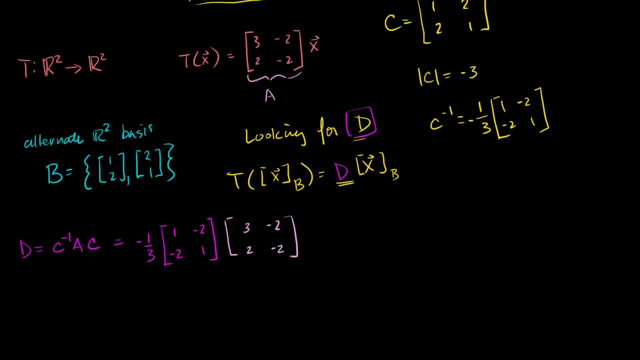 Times c. c is right there. I'll do it in yellow Times c, which is 1,, 2, and then 2, 1.. So let's do this piece by piece, Let's work through this. So what is this piece going to be equal to? 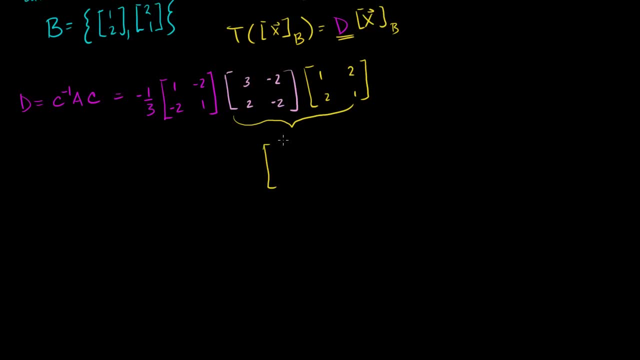 We have a 2 by 2 times a 2 by 2.. That's going to give us another 2 by 2 matrix. So this first term right here is going to be 3 times 1 plus minus 2 times 2.. 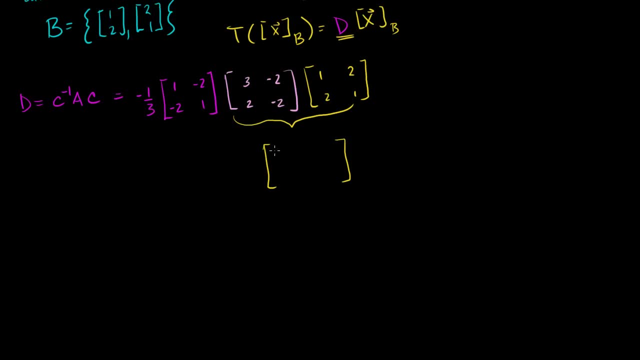 So 3, 3 minus 4.. So it's going to be minus 1.. 3 times 1 plus minus 2 times 2.. Right, it's minus 1.. Then you have 3 times 2, which is 6, minus 2.. 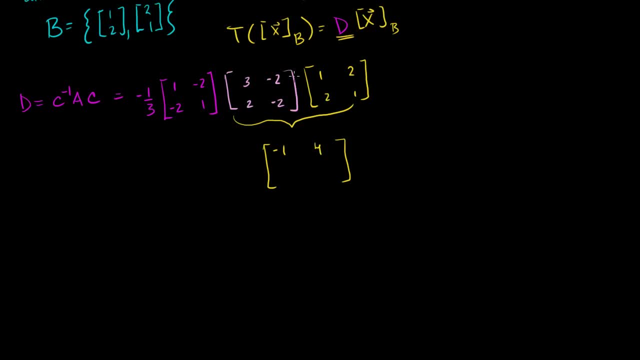 Right minus 2 times 1.. So that is 4.. Right 3 times 2.. Right 3 times 2 minus 2 is 4.. And then, when you go down here, 2 times 1 minus 2 times 2.. 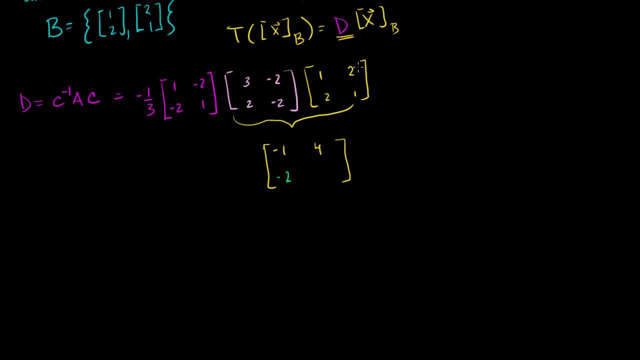 That's 2 minus 4.. That's minus 2.. And then 2 times 2 is 4 minus 2 times 1.. So 4 minus 2 is just 2.. So our matrix D is going to be equal to minus 1 third times. 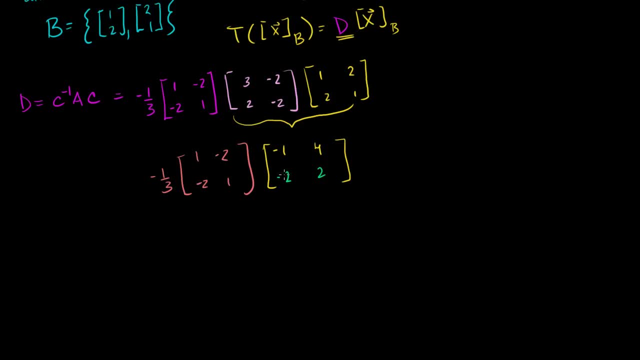 this guy, 1 minus 2 minus 2, 1, times this guy, which was just the product of those two matrices. Now let's figure out what this is. If I take the product of these two guys, it's going to be: 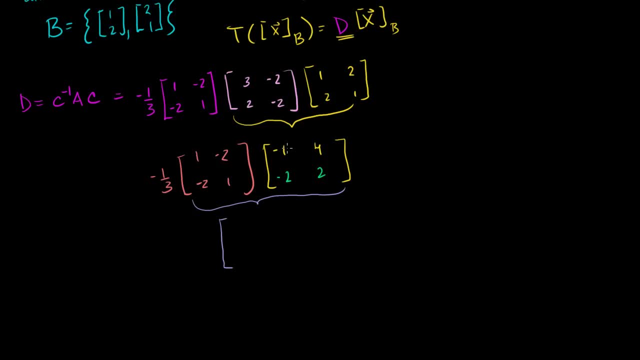 another 2 by 2 matrix. So I have 1 times minus 1,, 1 times minus 1, which is minus 1, plus minus 2 times minus 2.. Minus, 2 times minus 2.. So let me make sure. 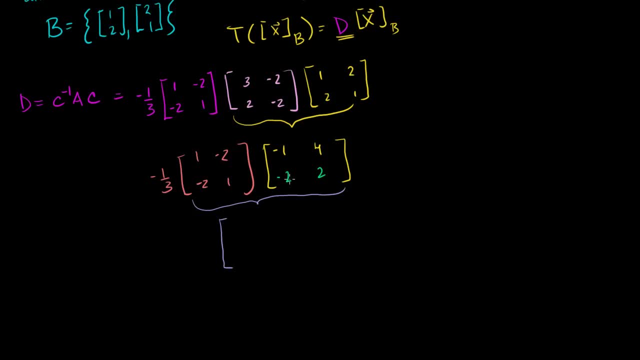 So 1 times minus 1, minus 2 times minus 2 is 4.. And then 1 times minus 1 is minus 1.. So it's going to be 3.. And then we have. and then we go to the next term. we have. 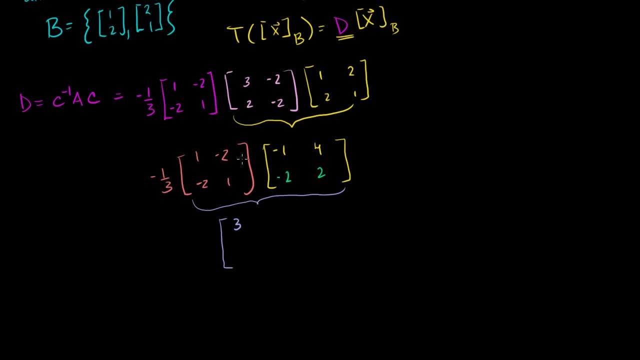 1 times 4.. Plus minus 2 times 2.. So that's 4 minus 4,, which is 0. And then we have minus 2 times minus 1,, which is 2, plus 1 times minus 2.. 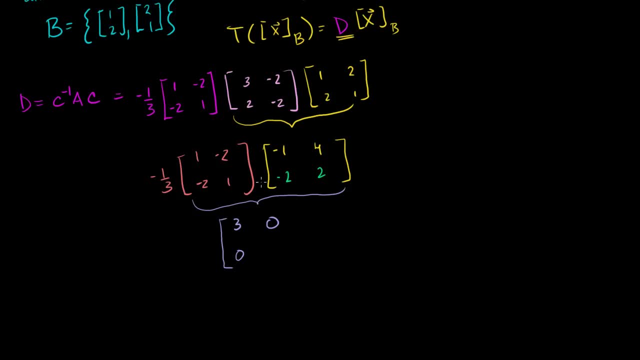 So that is 0.. And then finally, we have minus 2 times 4, which is minus 8, right? Minus 2 times 4 is minus 8, plus 1 times 2.. So minus 8, minus 2 times 4 is minus 8, plus 2 is minus 6.. 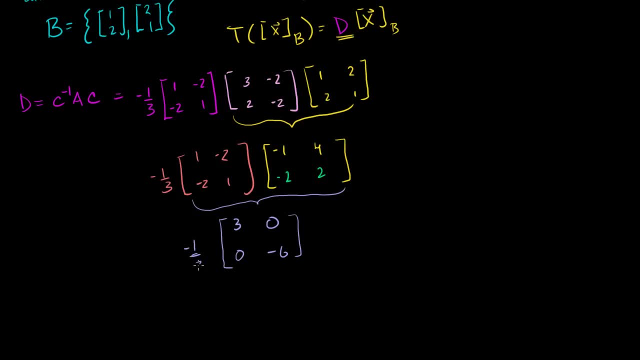 And all of that times minus 1 third. So this is going to be equal to 3 times minus 1. third is minus 1, 0, and then 0. Minus 6 times minus 1. third is 2.. 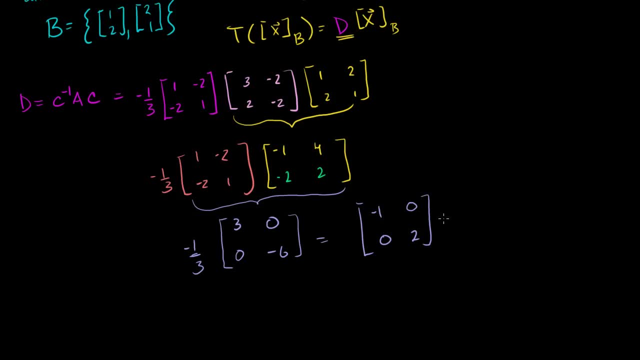 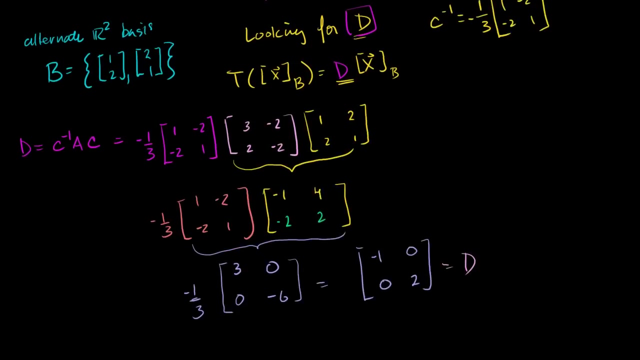 So this is so. D is now our transformation matrix with respect to the basis B, With respect to the basis B. So we were able to figure it out Just applying this formula here. Now what happens? let's actually do it with some. 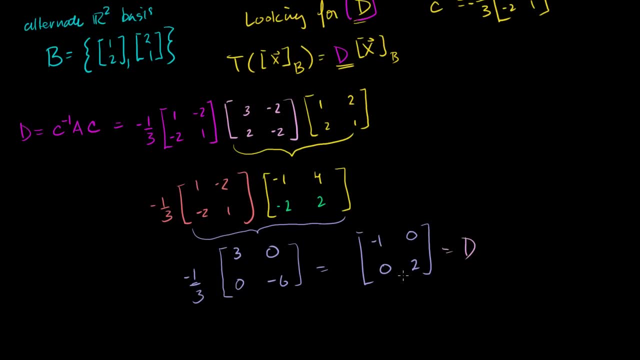 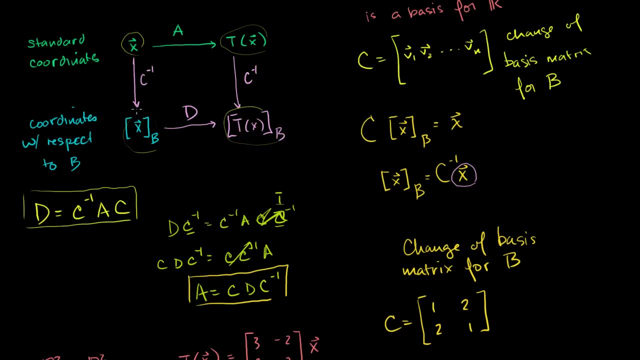 actually I'll save that for the next video where we actually show that it works, That we can actually take some vectors. we can actually take some vectors x, apply the transformation or apply the change of coordinates to get to this, and then apply D and 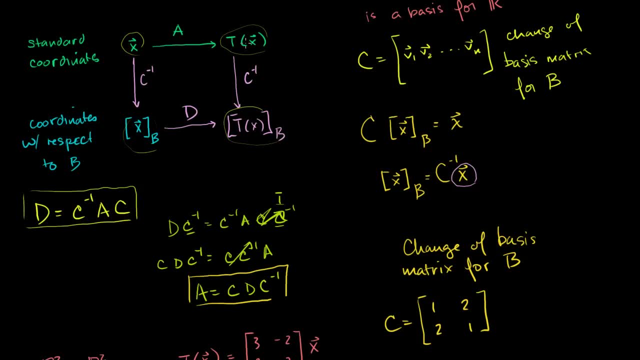 then maybe we could go up that way: multiply by C to get the transformation. It's going to be equivalent to A. I'll do that in the next video. 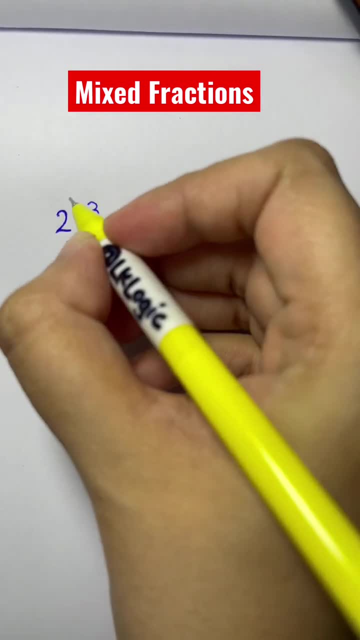 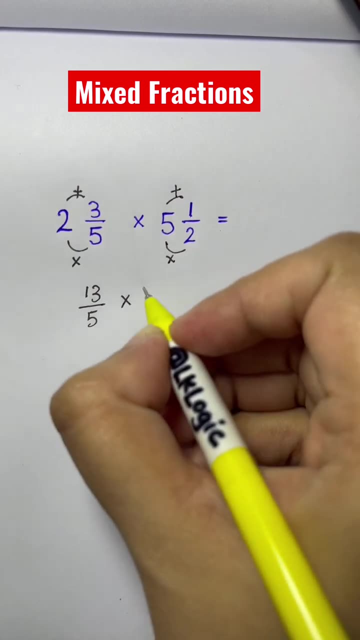 how to multiply two mixed numbers. just convert it first: 5 times 2 is 10, 10 plus 3 is 13- 13 over 5. and this one 2 times 5 is 10. 10 plus 1 is 11- 11 over 2. now multiply the denominators 5 times 2 is: